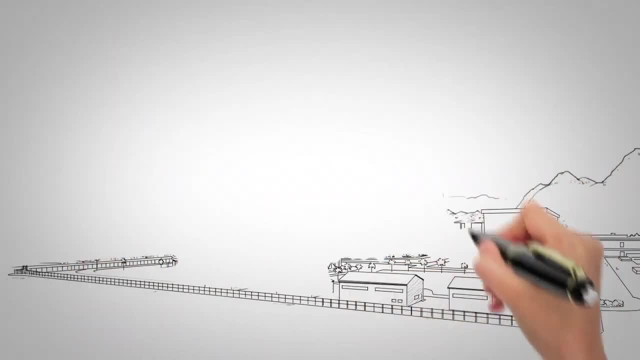 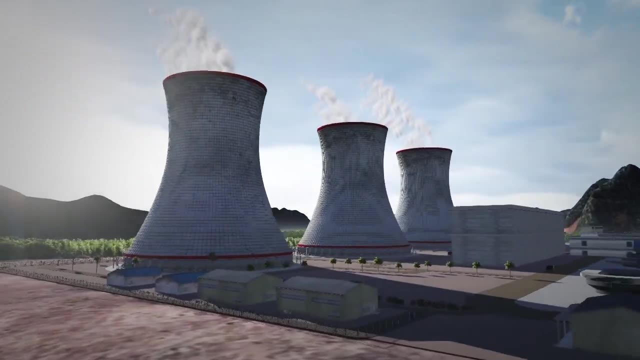 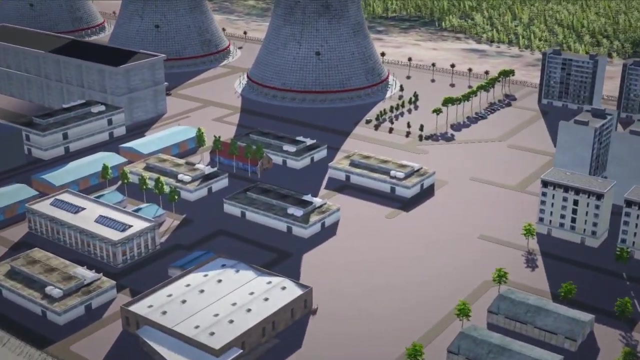 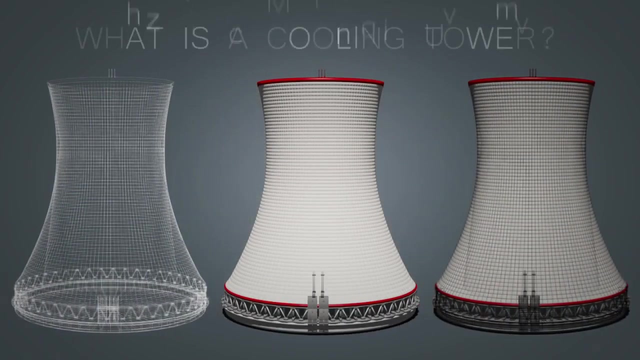 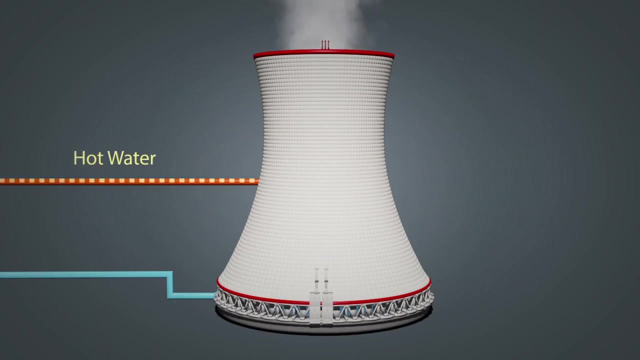 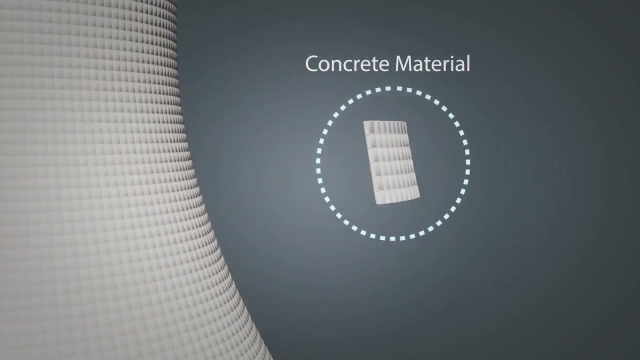 Cooling Tower. When we see a nuclear power plant, we can easily distinguish the cooling tower Cooling Tower. Cooling Tower is the place the coolant medium of water is cooled down for reusing it in the power plant. In this concrete structure, hot water is allowed to cool down, thereby releasing the thermal energy into the environment. 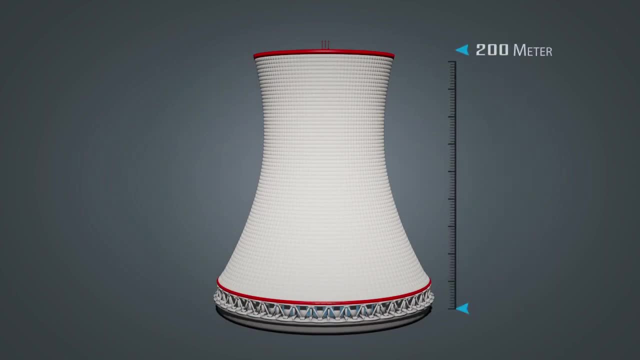 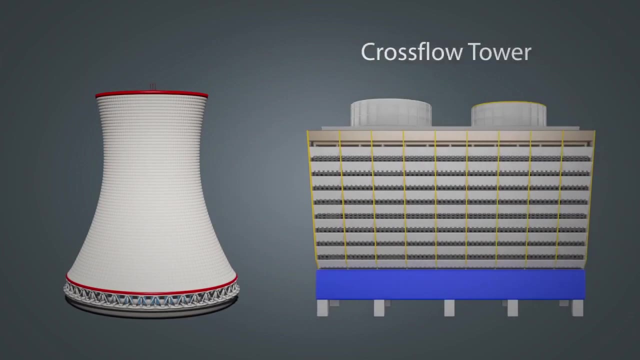 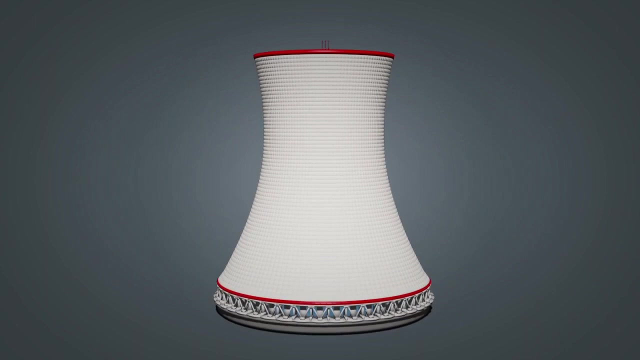 The cooling tower can be up to 200 meter tall. There are two types of cooling towers. One is cross flow type and the other is counter flow type. Before moving on to the working of a cooling tower, let us look at the components of a counter flow type cooling tower. 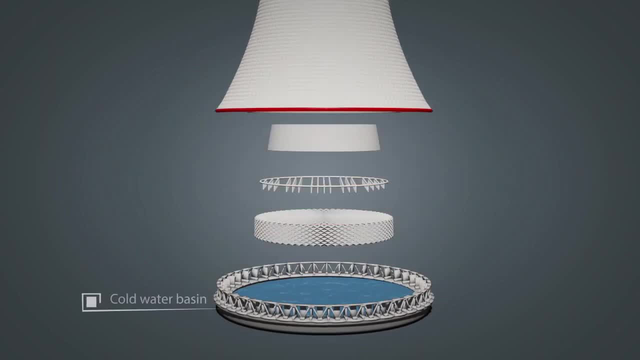 A counter flow type of tower has cold water basin, air inlet, fill media, spray nozzles and drift eliminator. Hot water is pumped into spray nozzles. Due to the natural convection, cold air gets drawn from outside through air inlet. 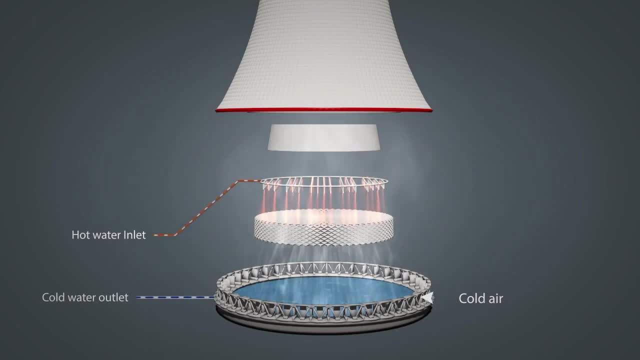 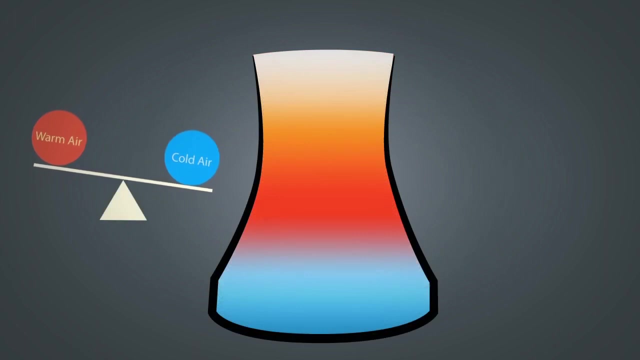 The cold air then cools down the water, which is stored at the very basement of the tower. Note that during this process, about two percent of water evaporates. A cooling tower works on the principle of natural circulation. Due to the difference in density, the warm air rises up and escapes from the opening at the top of the tower. 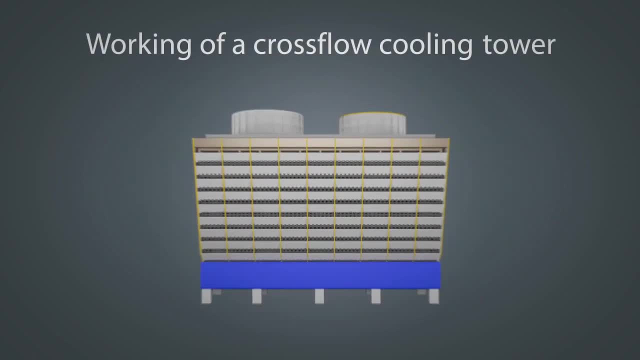 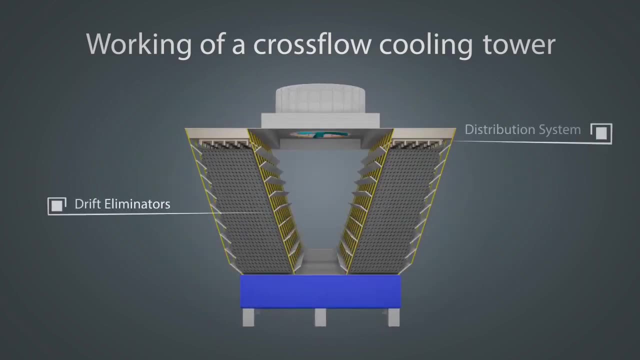 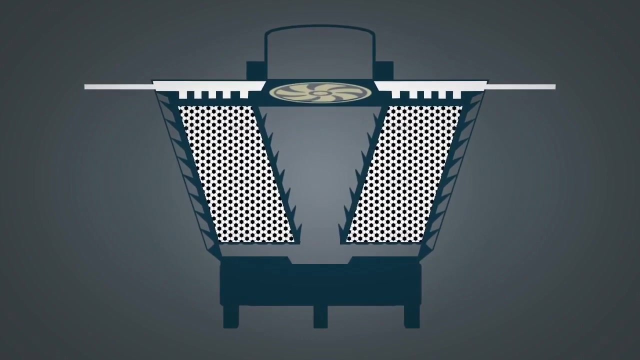 Now let's understand the components and working of a cross flow type cooling tower. This type of cooling tower has drift eliminators, distribution system, fill media and exhaust fan. In case of a cross flow cooling tower, hot water is sent through a water inlet to the cooling tower. 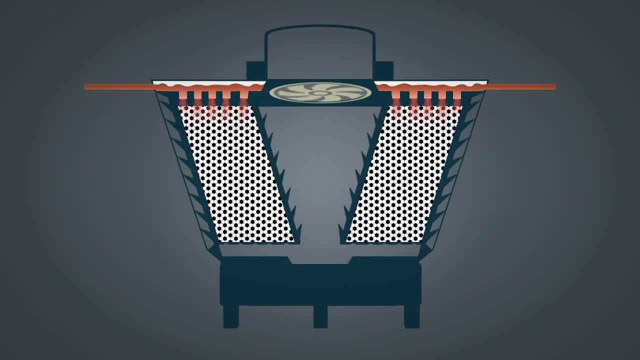 Then it is distributed on the fill media through water distribution system. The gravity causes the water to cascade down across the fill media. The fill media breaks the water stream into smaller water droplets, creating a large surface area for heat transfer. Using baster and hopper, a particular type ofhões is set for up to inner lack of water.